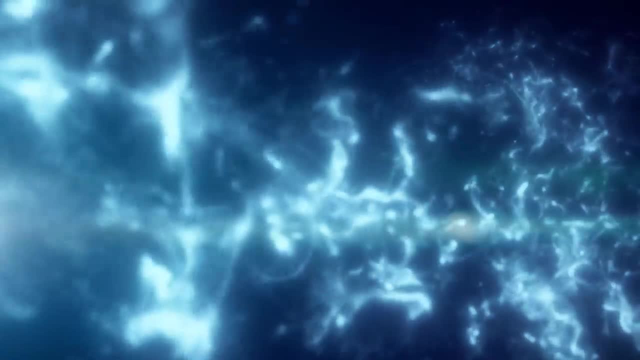 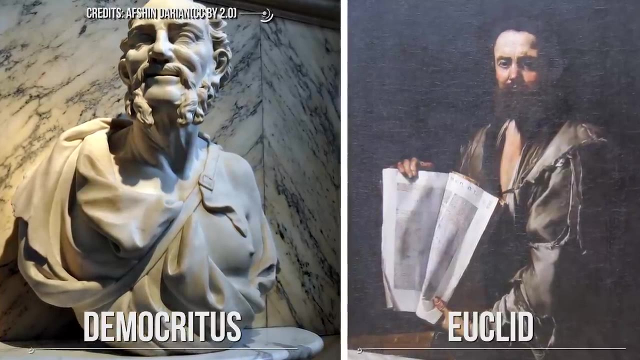 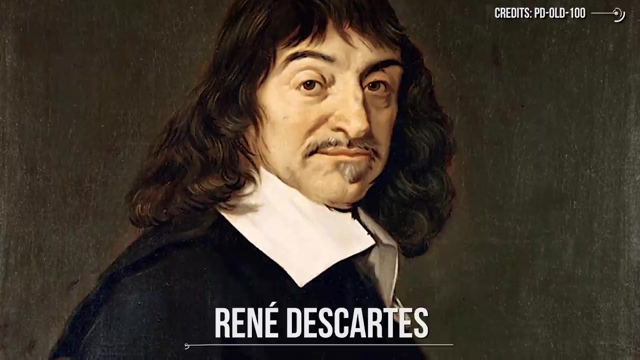 different researchers have expressed themselves about the nature of light in the course of history. Even if some theories were elaborated by great Greek thinkers like Democritus or Euclid, the major contributions were made in the 17th century. Firstly, in 1630, the famous René Descartes popularized and accredited the wave description. 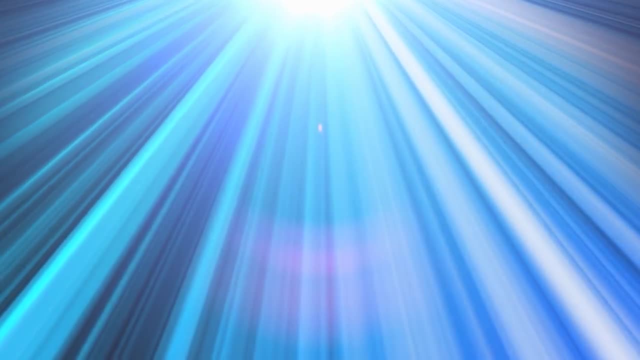 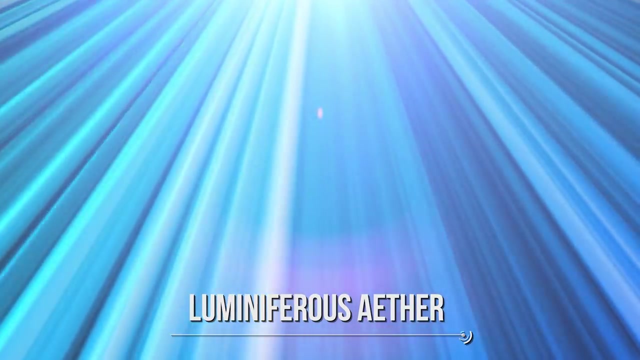 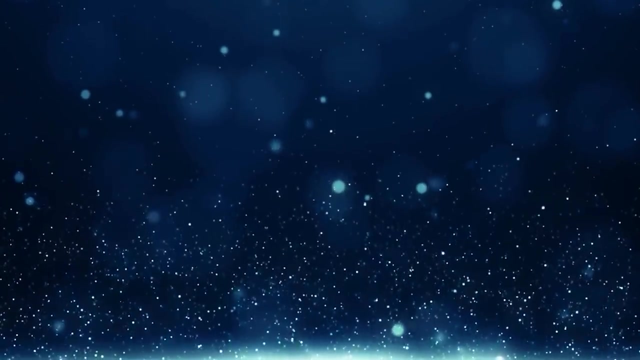 in his treatise on light, the world showing that the behavior of light could be recreated by modeling wave-like disturbances in a universal medium called luminiferous ether. Some years later, a brilliant British physicist developed and documented an opposite theory that described light as a particle. Want to know his name. 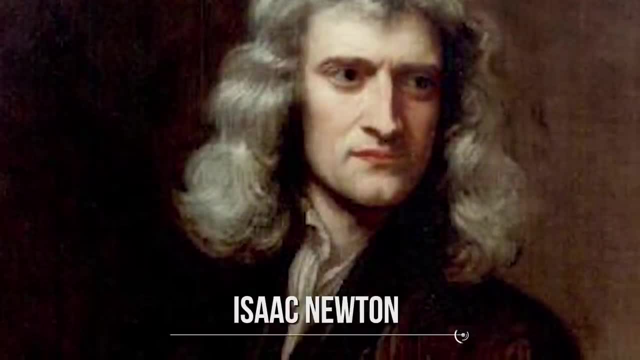 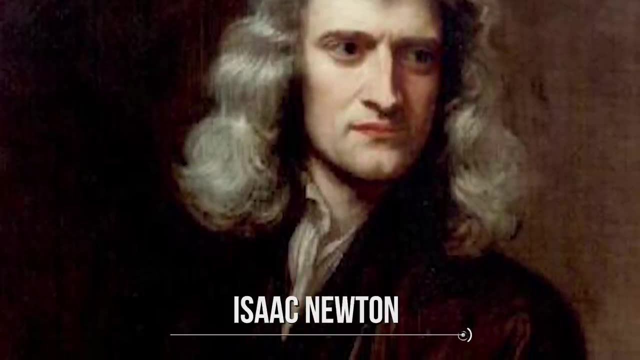 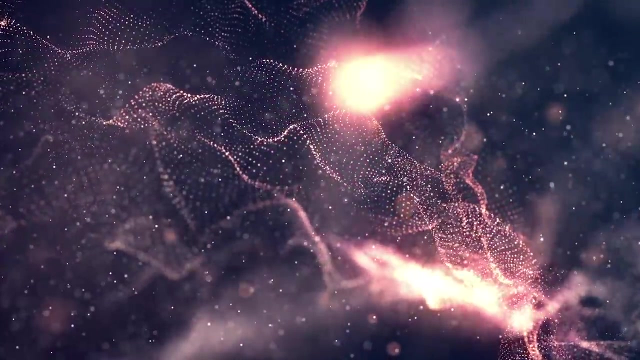 Isis Newton. Starting in 1630,, Sir Isaac studied for three decades the behavior of this incredible thing called light, which allows us to see the entire world. The British scientist defined rigorously the effects of reflection and refraction. He understood that the angle of incidence is the 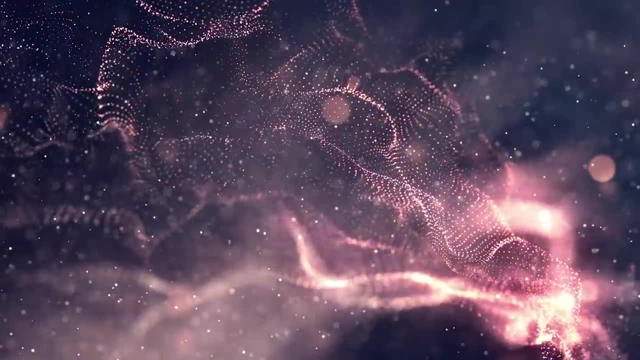 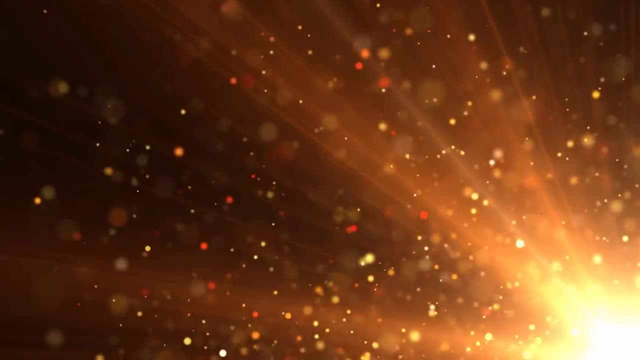 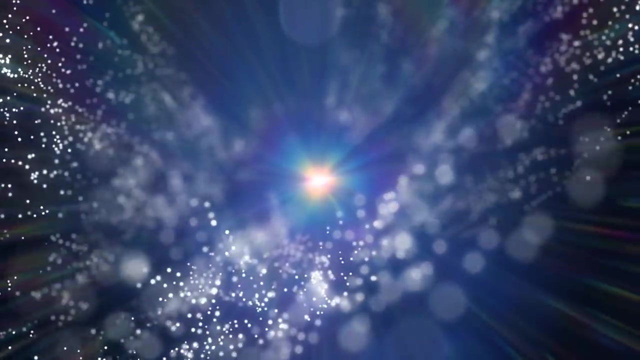 same of the angle of reflection, which is practically the same behavior of a particle that hits a rigid wall. By observing these phenomena, Newton came to the conclusion that light was definite light, Definitely considerable, like a particle. He developed and championed his corpuscular theory, arguing that the perfectly straight 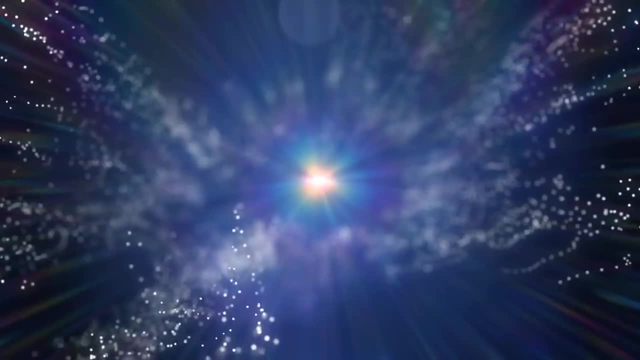 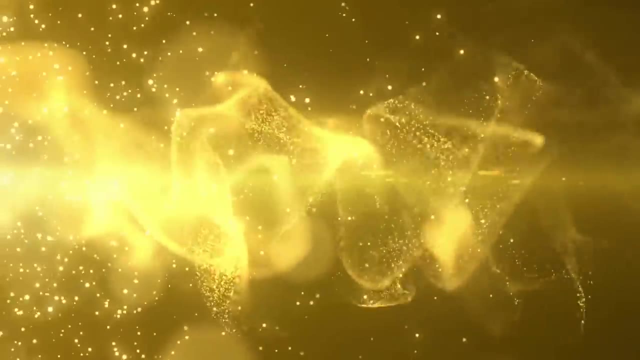 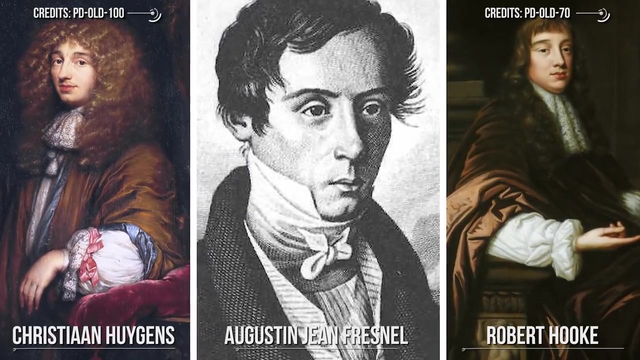 lines of reflection demonstrated light's particle nature. Only particles could travel in such straight lines. He explained refraction by positing that particles of light accelerated laterally upon entering a denser medium. Meanwhile, other famous scientists like Christian Huygens, Augustin Jean Fresnel and Robert Hooke elaborated the concept of wave by. 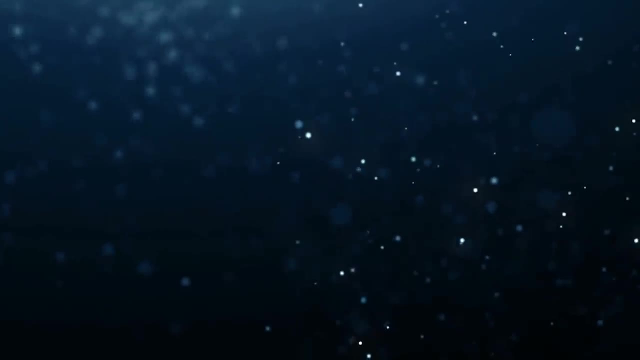 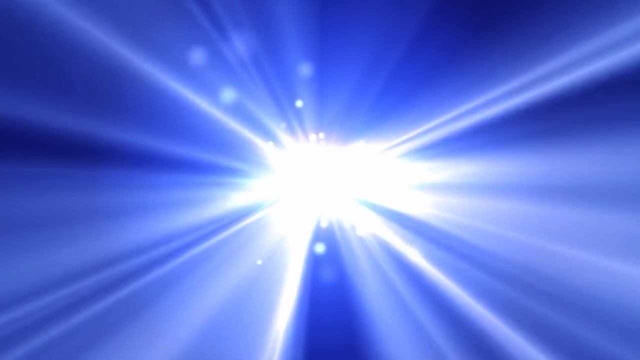 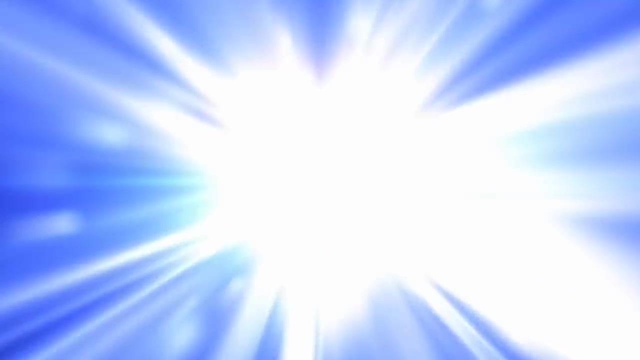 using mathematical tools, and they discovered that both reflection and refraction could be explained through this model. It was born of the wave theories of light. The different speed in different materials could be easily derived as a consequence of the medium-dependent propagation of waves. Around one century later, an experiment carried out by Thomas Young in 1801, 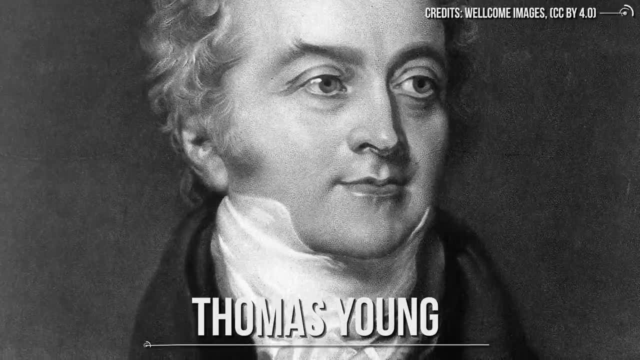 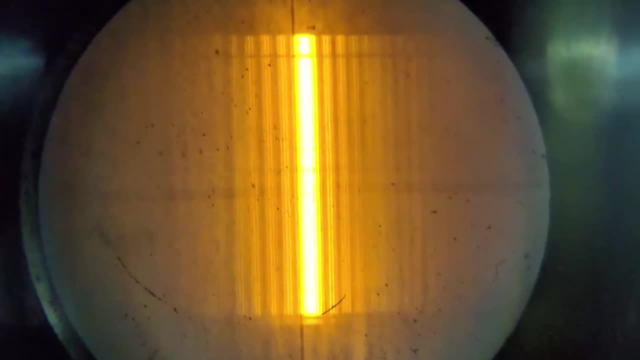 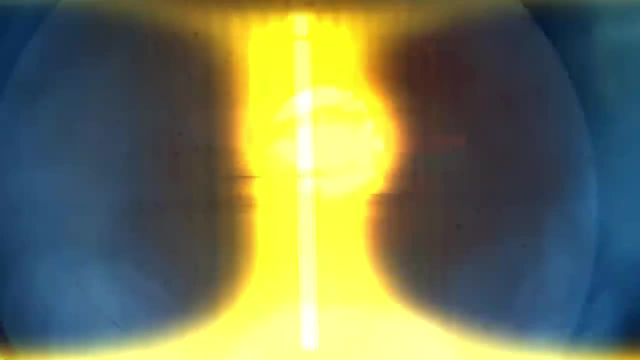 apparently ended the debate regarding the wave-particle duality of light, the double-slit experiment. What was it about? Let's start with a more simplified version called the single-slit experiment. It's based on firing light through a slit that allows it to reach a screen If light consisted strictly. 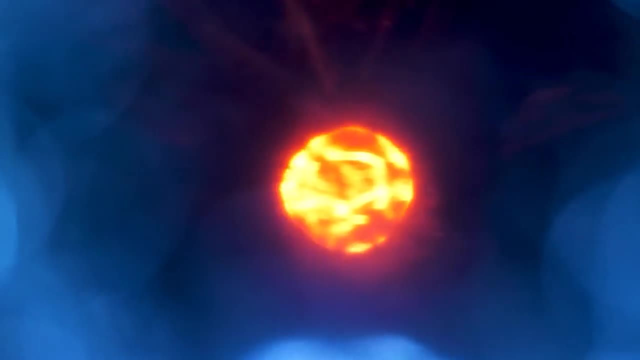 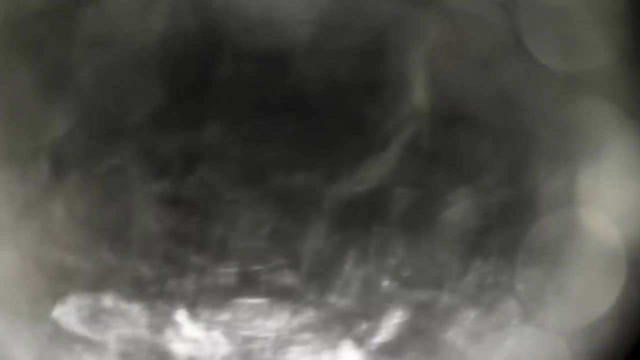 of ordinary or classical particles, we would expect to see a pattern corresponding to the size and shape of the slit. However, when this single-slit experiment is actually performed, the pattern on the screen is a diffraction pattern in which the light is spread out. 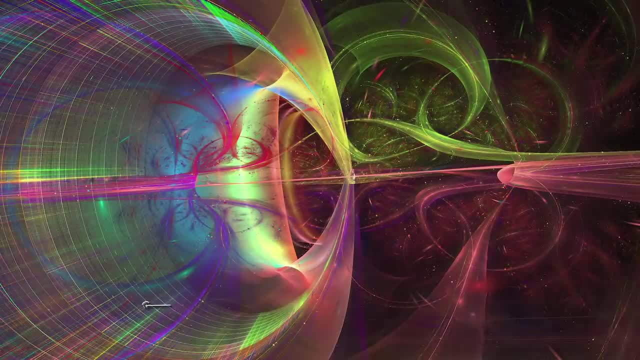 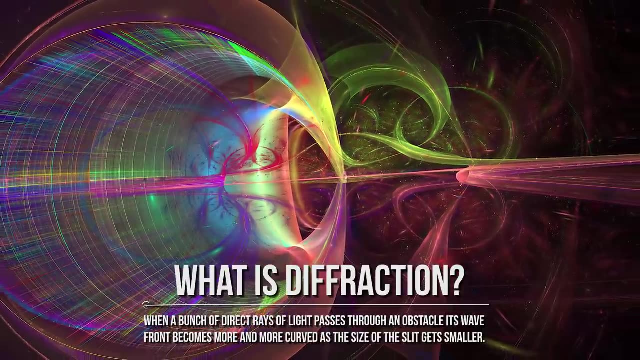 The smaller the slit, the greater the angle of spread. What is diffraction? When a bunch of direct rays of light passes through an obstacle, its wavefront becomes more and more curved as the size of the slit gets smaller. To be more precise, 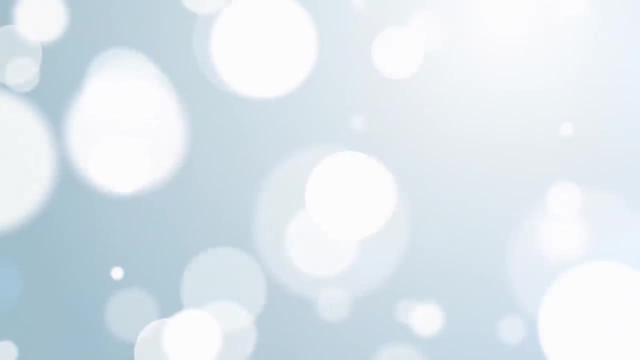 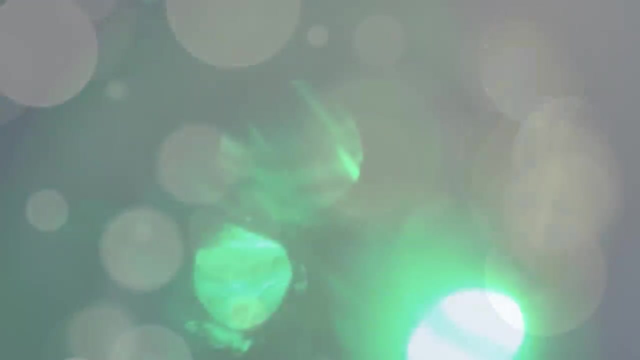 the rays that pass into the slit interferes with each other, generating a spherical wave. It's a very interesting phenomenon that we can even see on sea waves, So this version of the experiment confirms the wavy nature of light. What happens if we use two? 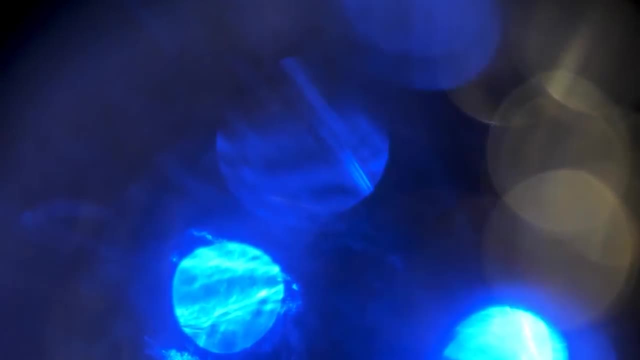 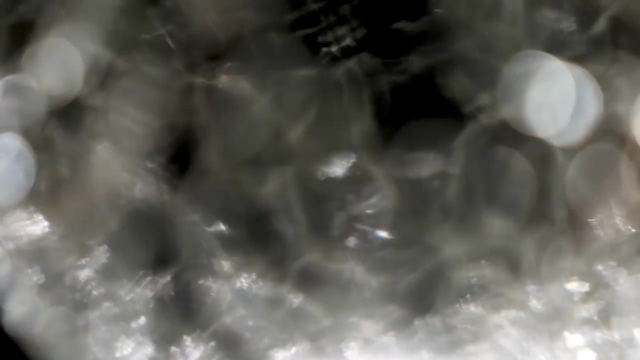 slits of the same size. The pattern on the screen gets more pronounced, with a series of dark and light bands. How can we explain this result? by using the properties of waves. Well, we have two curved wavefronts, similar to the one of the single slit. 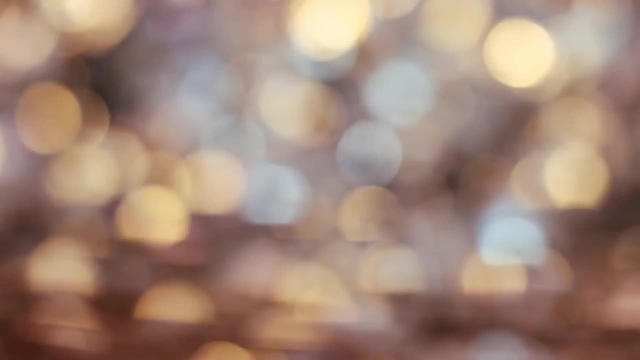 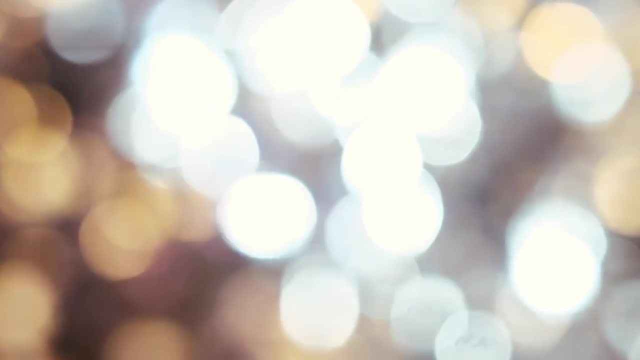 but this time they interact with each other. We have a case of interference. in some regions this interaction will be constructive, amplifying the intensity of light, Whereas in others it will be destructive: the waves cancel out each other. 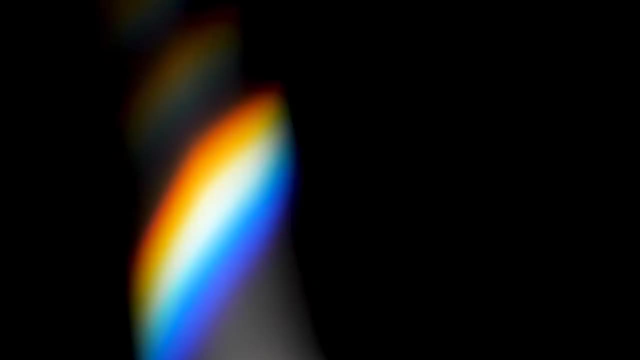 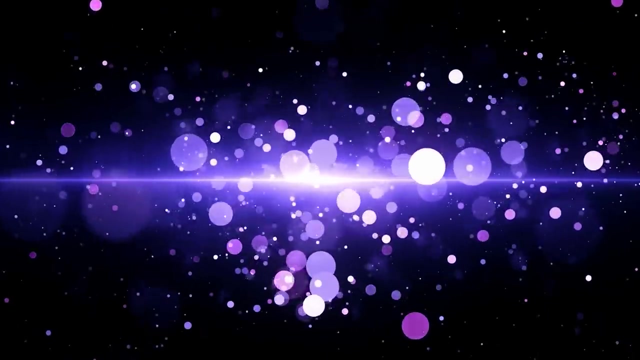 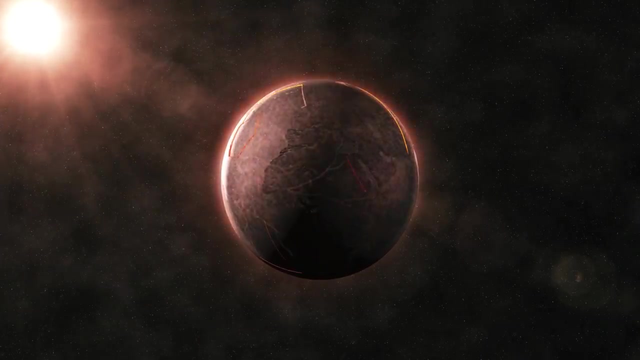 saying before, this experiment made scientists refuse Newton's corpuscular ideas and ended the debate regarding the wave-particle duality of light. However, in the 19th century, something really incredible for physics totally changed the perspective on this topic. Before finding out more about this, be sure to like or dislike the video. 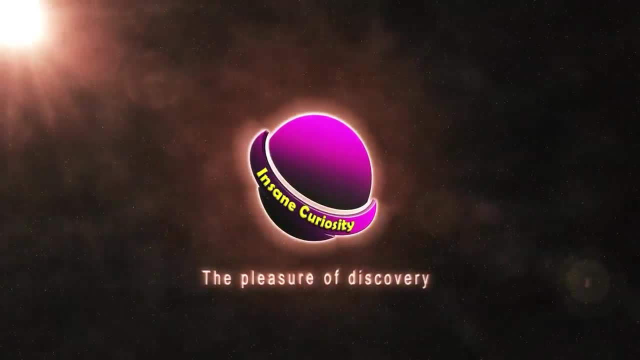 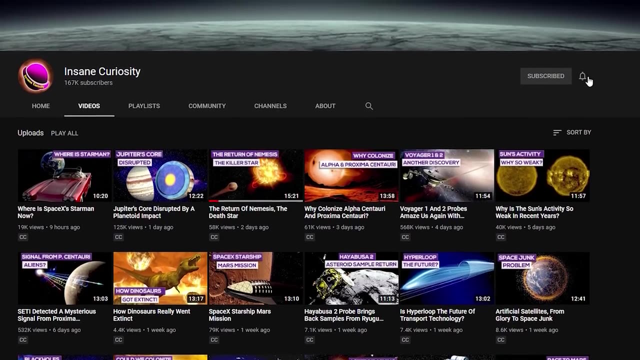 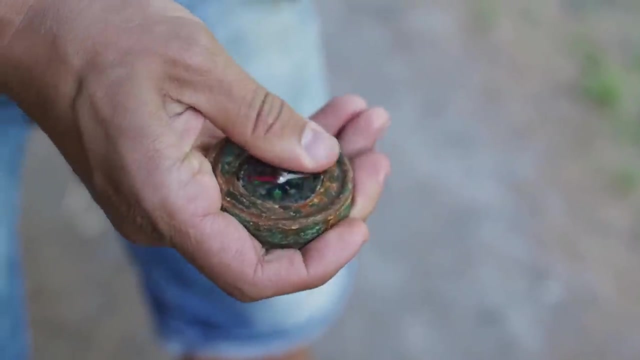 so that we can continue to improve and make these videos better for you, the viewer Plus. be sure to subscribe to the channel clicking the bell, so that you don't miss any of our weekly videos. Physicists observed that electric wires interacted with each other and slight changes in current made. 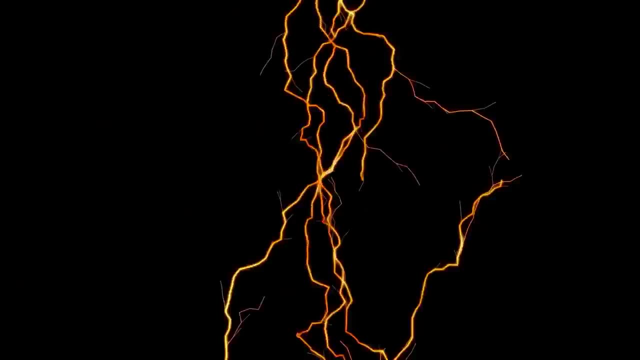 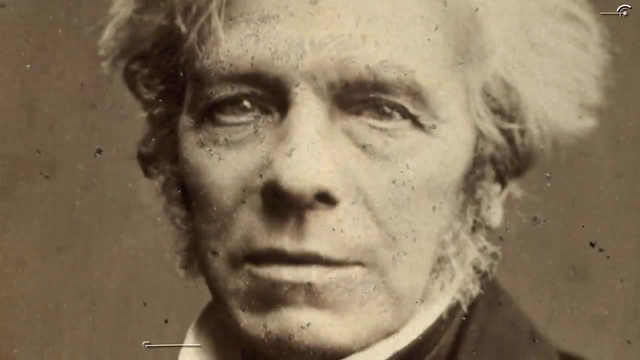 magnetic compasses turn around. Briefly speaking, they understood that electricity and magnetism were two different aspects of one unique interaction: electromagnetism. Although the major experiments and laws were elaborated by Faraday and Henry- the man who gave the major 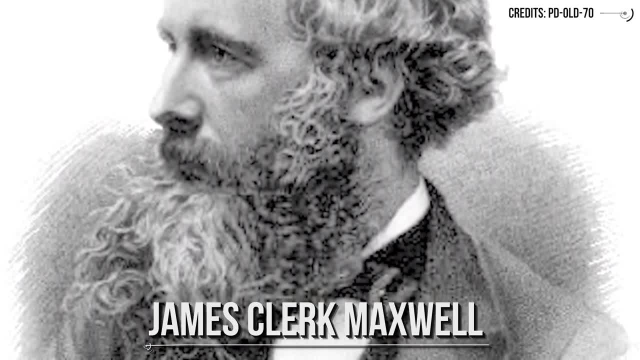 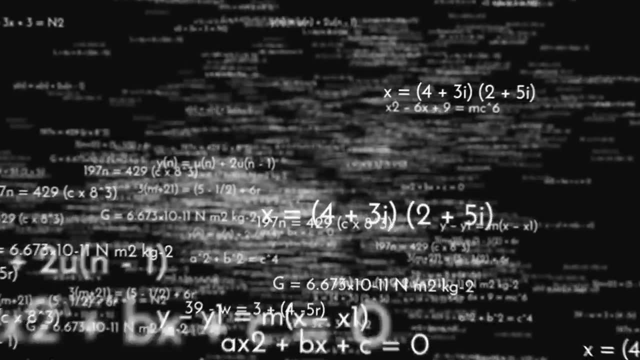 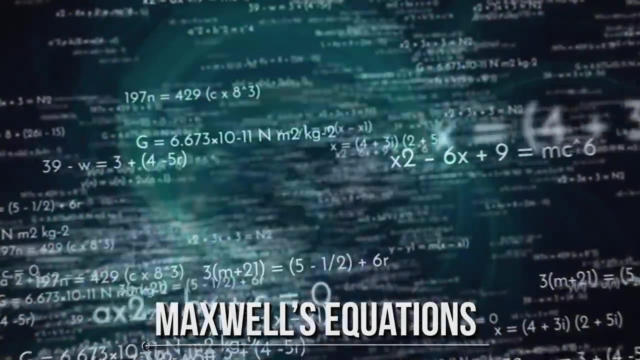 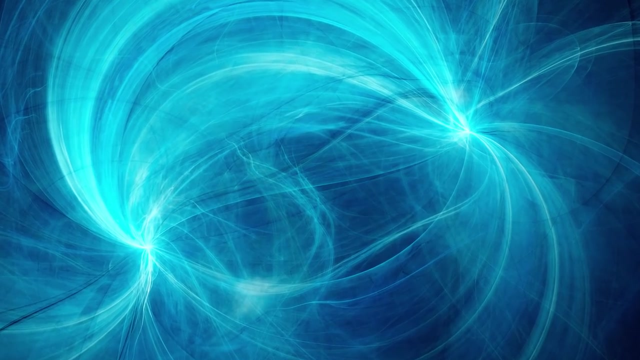 contribution to the development of electromagnetic theory was James Clerk Maxwell. He reunited all the precedent discoveries into four equations named after him, the Maxwell equations. These laws show that the two different phenomena can be united in one single theory. Moreover, these equations can be reassembled to produce what is known as a wave equation, both for the electric 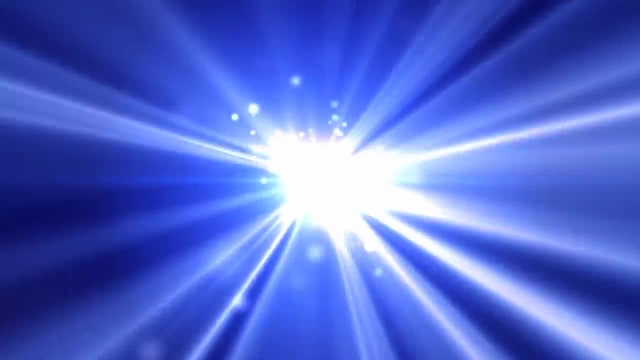 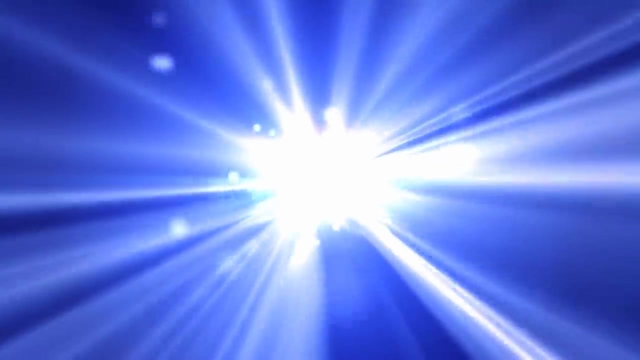 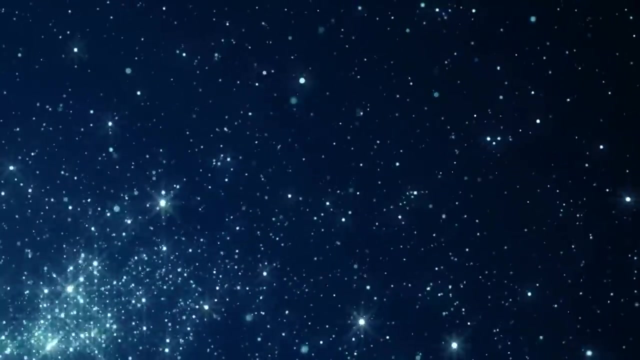 and magnetic field. The result of Maxwell's theory was the discovery of electromagnetic radiation that travels at the speed of light in different medium and even in empty space, differently from sound waves that need a medium to propagate. This fact was phenomenal, as all optics could be derived from that model, and it was another confirmation for the debate regarding 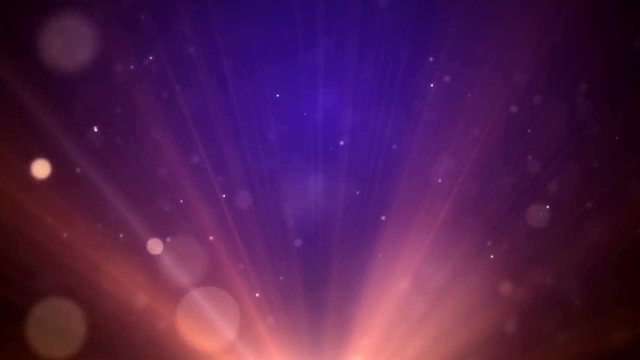 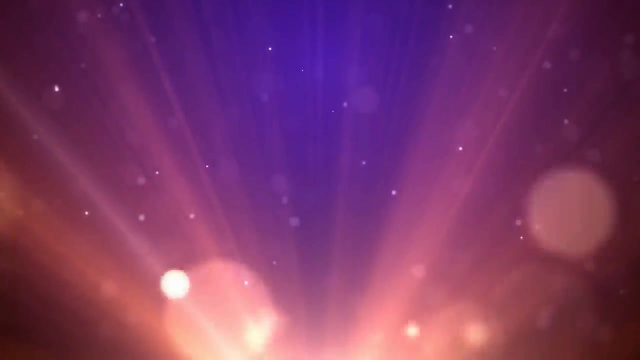 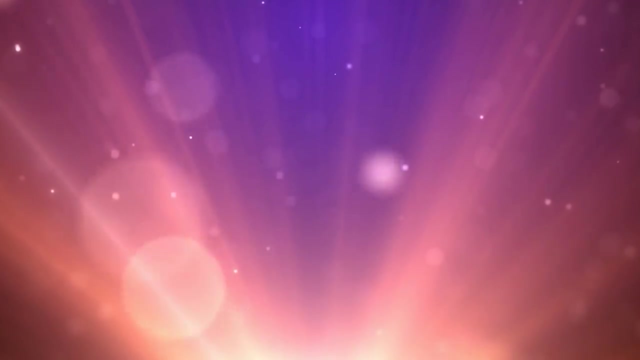 the wave-particle duality of light. At this point of history, physicists thought that our entire world could be described just by using gravity and electromagnetism that reproduce perfectly the experimental results. Some scientists even discussed if humanity had reached the end of physics research. But some important discrepancies in the description of effects. 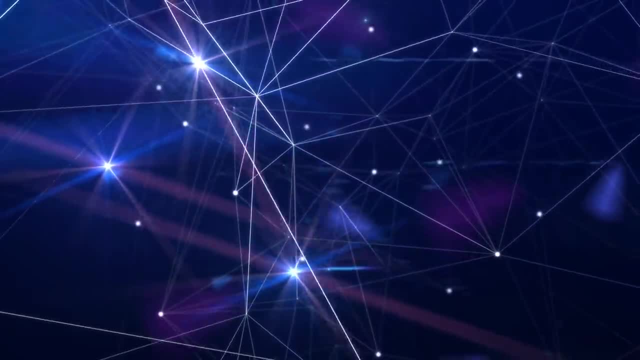 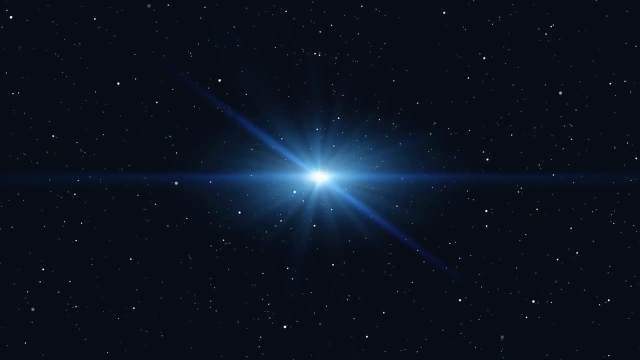 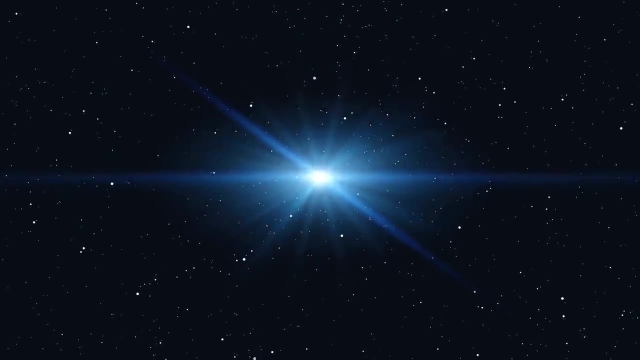 of metals totally revolutionized both the way of thinking about matter and the opinions regarding the wave-particle duality of electromagnetic radiation. What are we talking about? Well, to go on with our journey, we need to talk about stars. Yes, it might be a bit surprising. 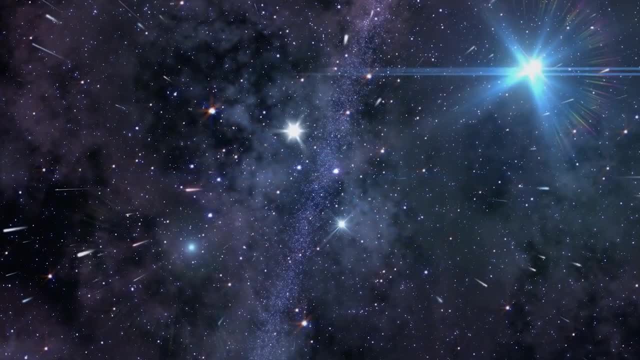 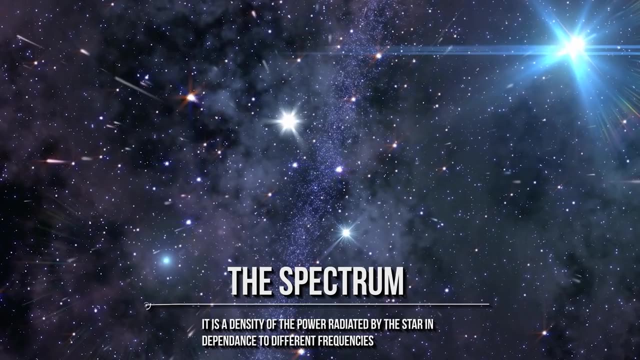 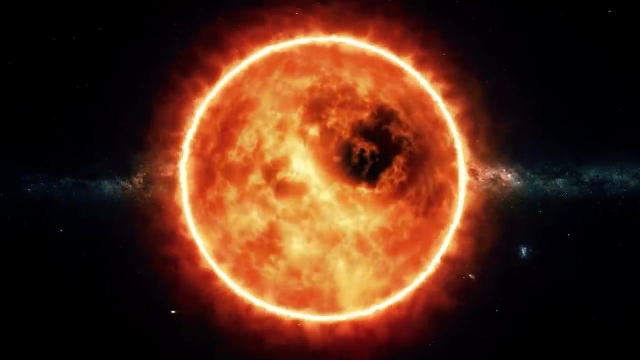 and confusing, but you'll understand everything later. Usually, astronomers analyze the emission of celestial bodies by studying the spectrum, which is a density of the power radiated by the star in dependence to different frequencies. More simply, the spectrum is a catalogue of the colors emitted by a star, The sun, for example. 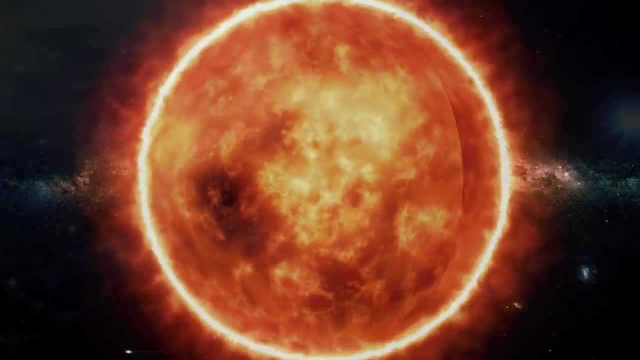 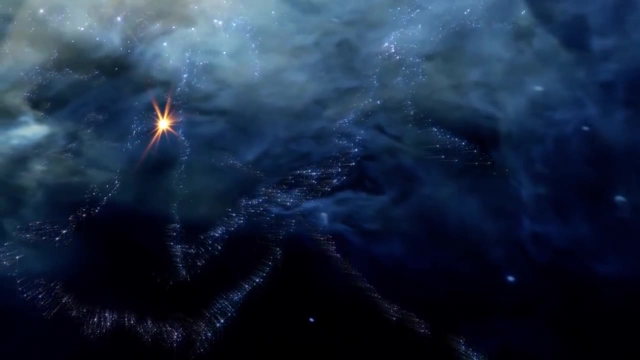 will have higher values of spectrum in the region of yellow and orange. The spectrum changes together with temperature. The most predominant frequency of emission is higher when the star is hotter. At the end of the 19th century, the main theoretical model used to classically describe this phenomenon 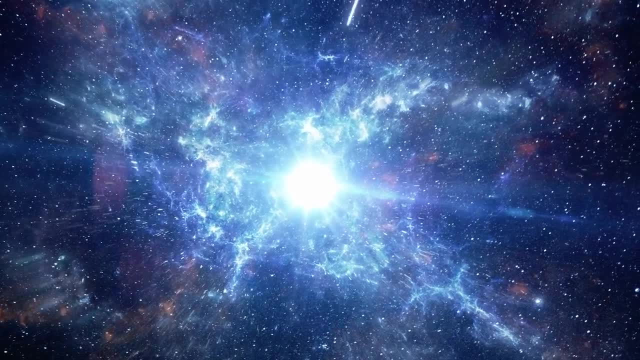 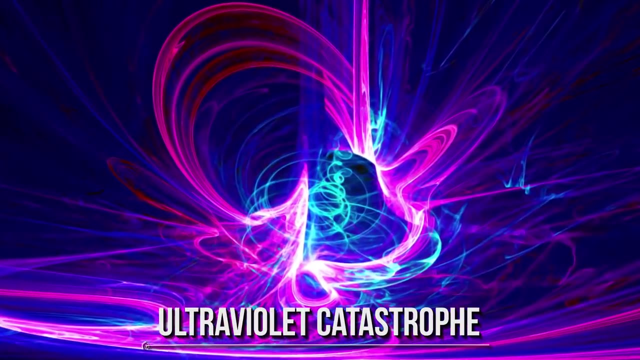 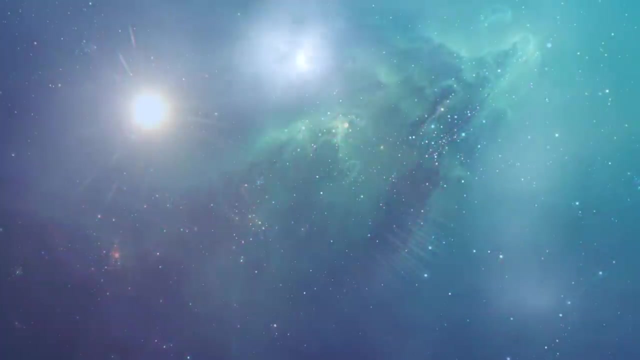 was named after Rayleigh, But it had a tremendous problem. It predicted that for very high frequency the emission was infinite. This topic was also known as the ultraviolet catastrophe, and it generated major concerns even in the public community. The only way to reproduce- 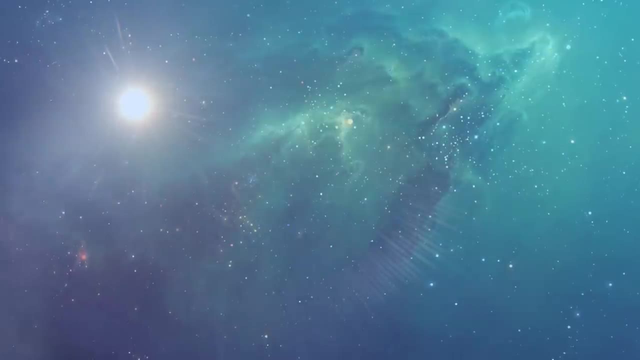 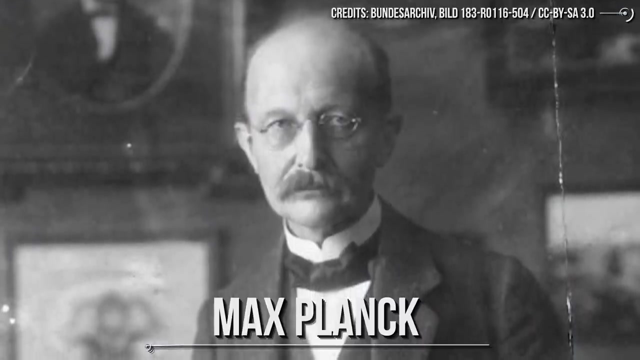 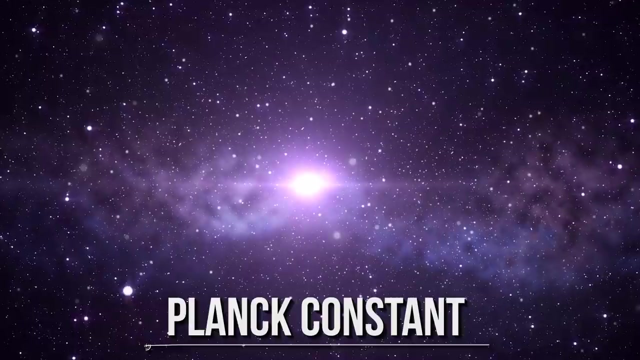 the experimental results that didn't have the spike before the violet region was developed by Max Planck. He proposed that the energy of a particle in the star was directly dependent on its frequency through a constant called Planck constant, as opposed to Rayleigh's model that was based on. 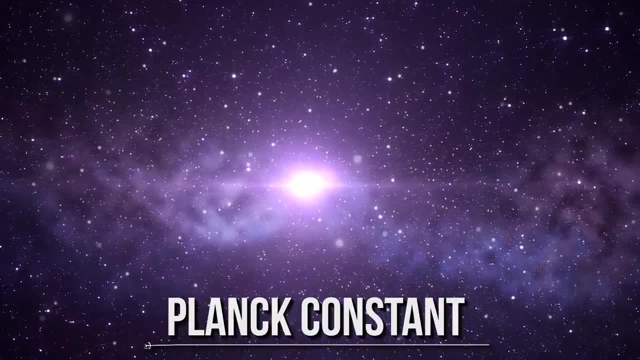 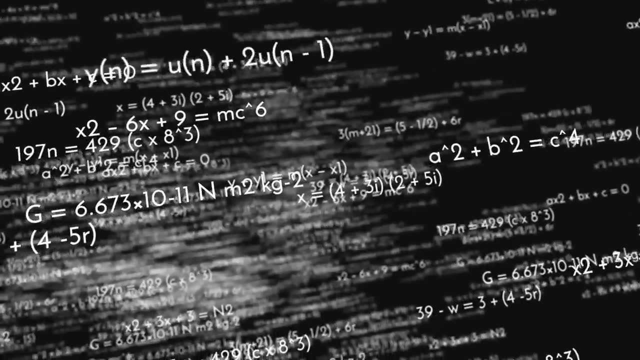 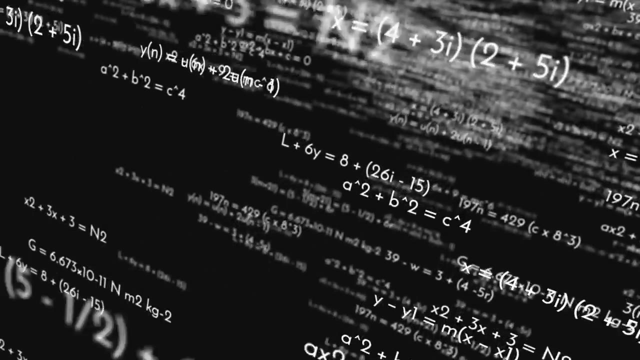 the dependence to temperature, Energy was proportional to temperature through the Boltzmann constant k. This mathematical adjustment was really strange and not rigorous, since it didn't have any theoretical foundation and physical meaning. however, these assumptions became crucial some years later. The second fundamental evidence was that the energy of a particle in the star was 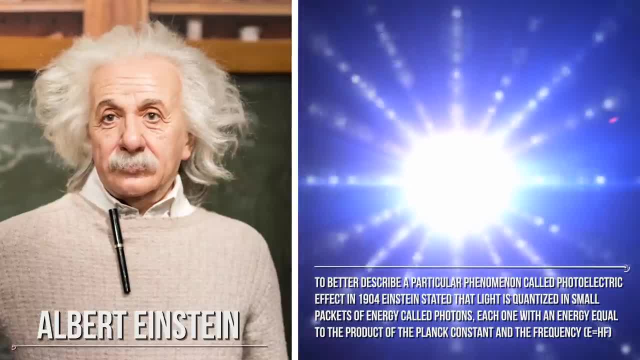 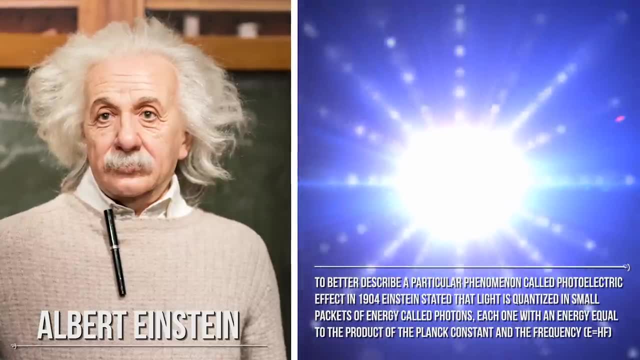 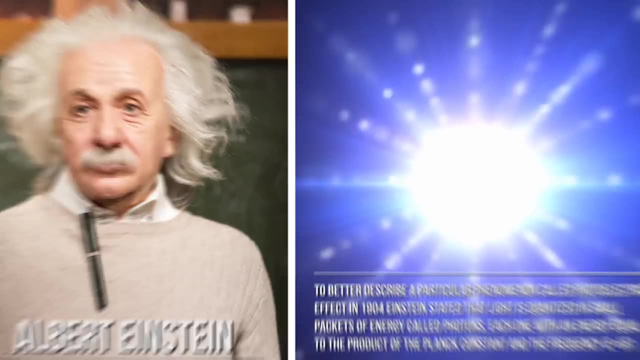 To better describe a particular phenomenon called photoelectric effect. in 1904, Einstein stated that light is quantized in small packets of energy called photons, each one with an energy equal to the product of the Planck constant and the frequency. What is this effect about? 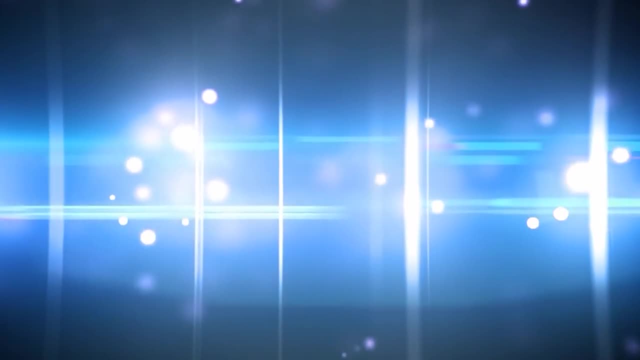 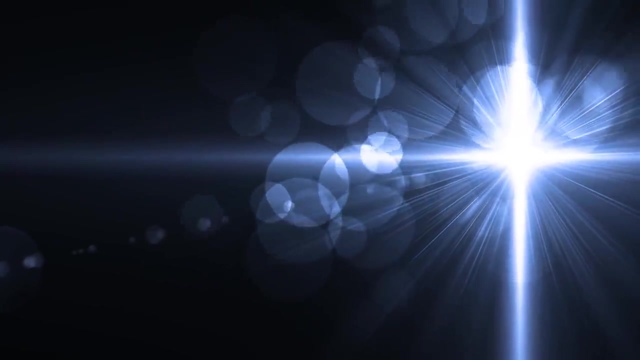 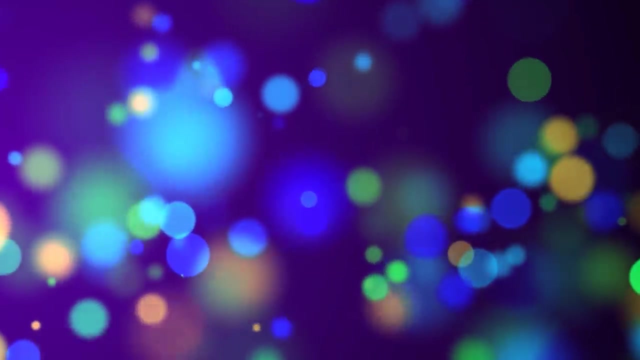 Photoelectricity is a property of some metals that emit electrons if stimulated by electromagnetic radiation. The classical predictions regarding this phenomenon were based on intensity: The more radiation on a metal, the more electrons could be emitted. However, experiments showed a different pattern. 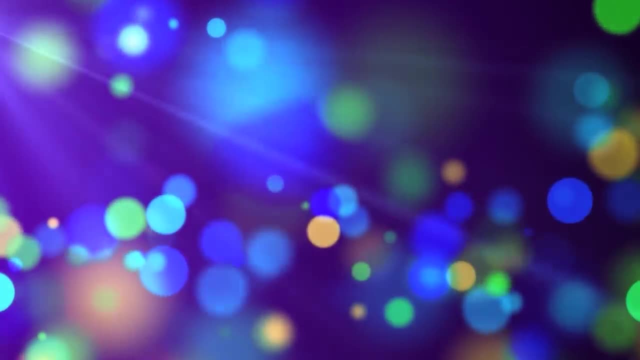 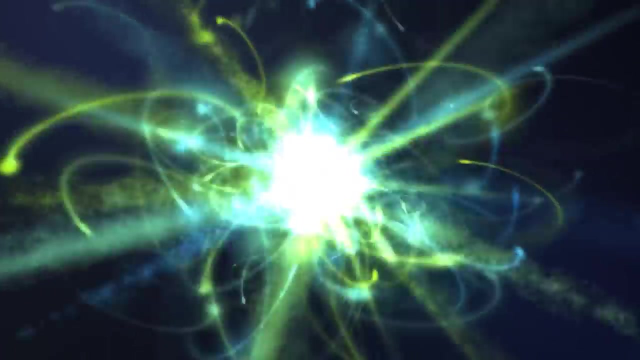 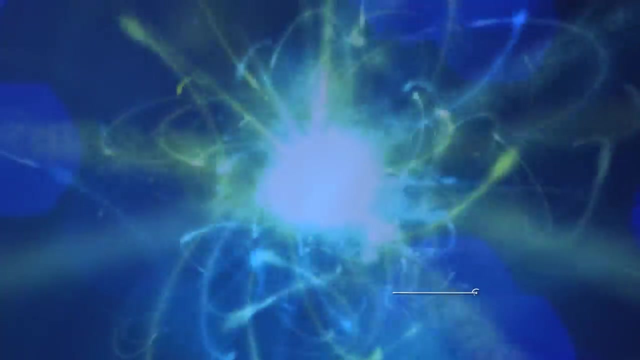 The emission just depended on frequency. Under a specific value, F0,, no electrons could be seen, and above that value, the relation between frequency and number of electrons was linear. If you double the frequency, the number of electrons emitted by the metal doubles. 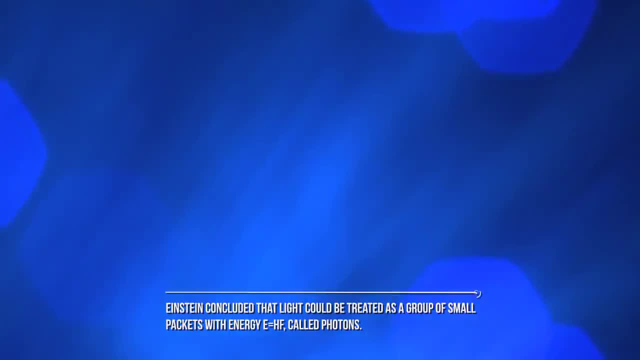 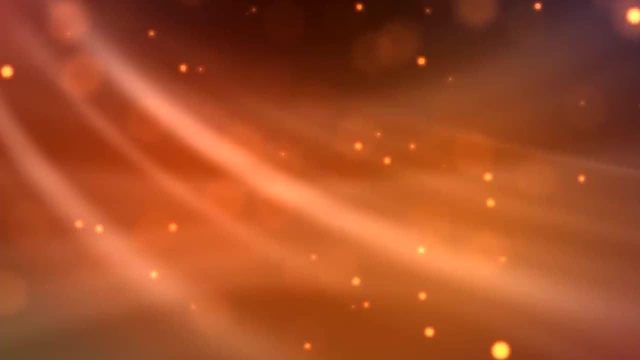 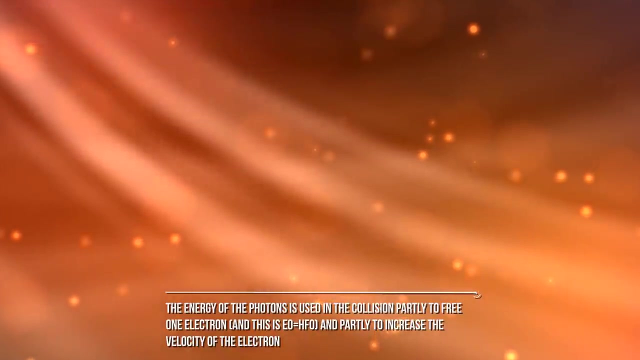 Einstein concluded that light could be treated as a group of small packets with energy E equals HF, called photons. They interact with electrons following the same laws of mechanical bodies. The energy of the photons is used in the collision partly to free one electron, and this is E0. 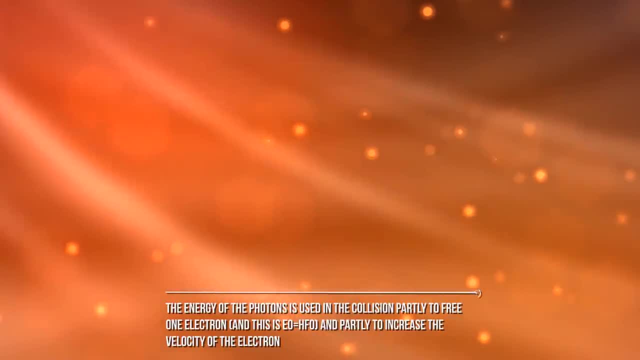 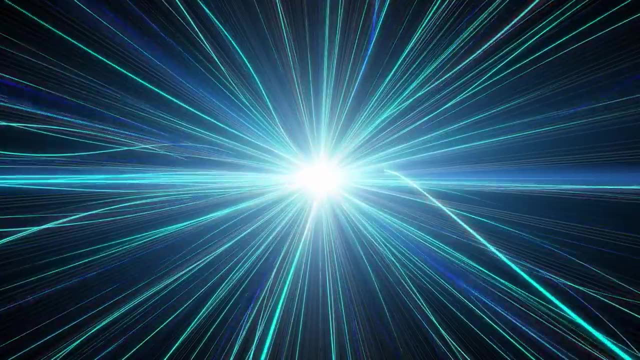 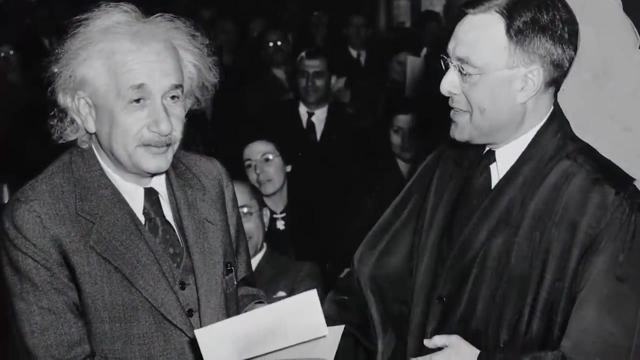 equals HF0, and partly to increase the velocity of the electron. If a radiation is more intense, it is composed by more photons. If an electron has a higher frequency, this means that each photon has a big energy. Thanks to this explanation of the photoelectric effect, Einstein received the Nobel Prize. 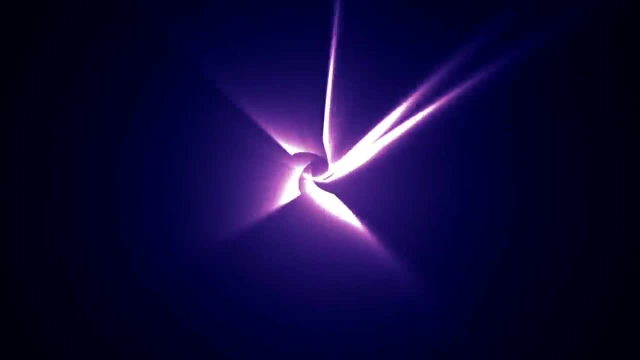 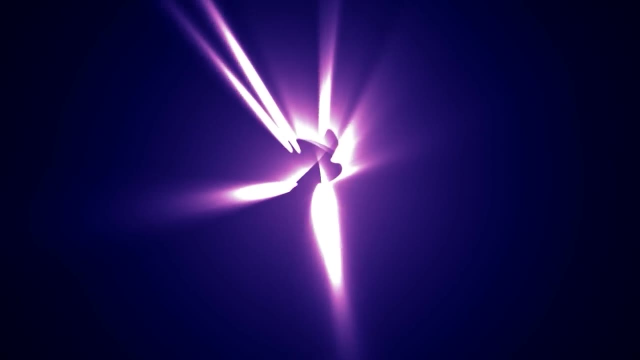 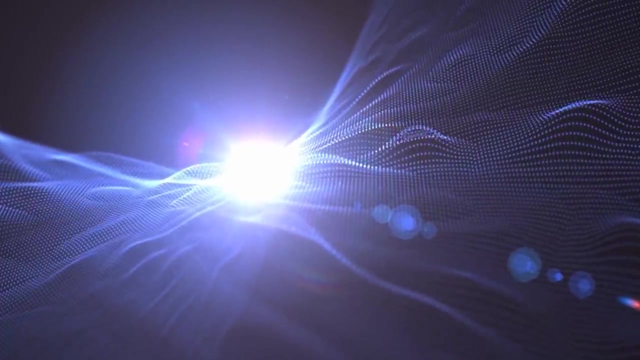 for Physics in 1921.. And it doesn't end here. With this discovery, Einstein made evident that energy emitted through electromagnetic radiation is quantized, and it's the beginning of quantum mechanics. This exciting model made physicists go crazy, as it revolutionized what they considered. 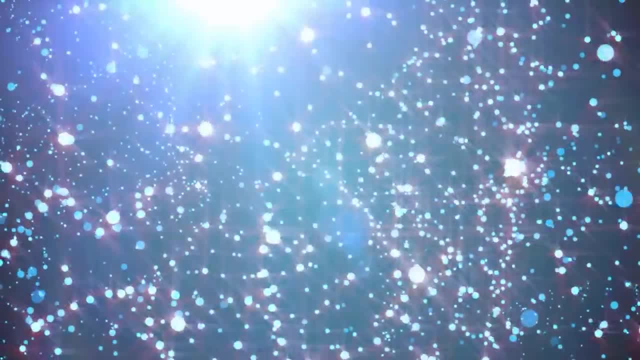 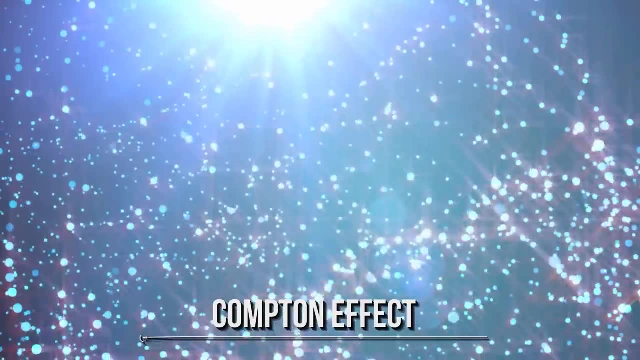 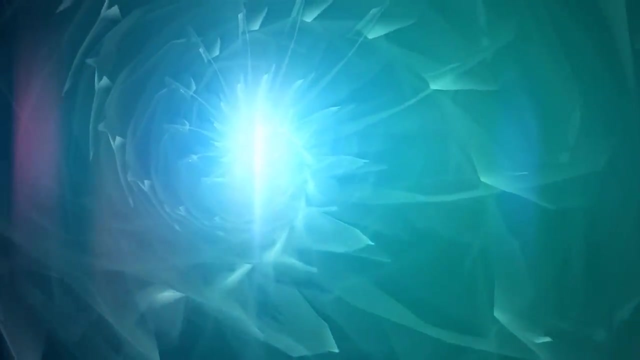 as a truth. The wavy nature of light. Einstein's discovery underlined that light can be treated also as a particle. Further studies on the so-called Compton effect confirm this hypothesis. But at the end, what is the solution to the wave-particle duality of light? 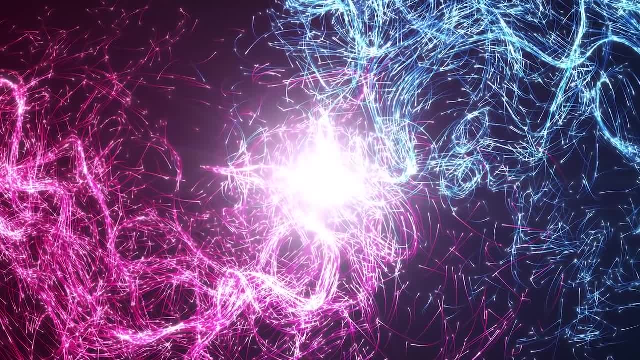 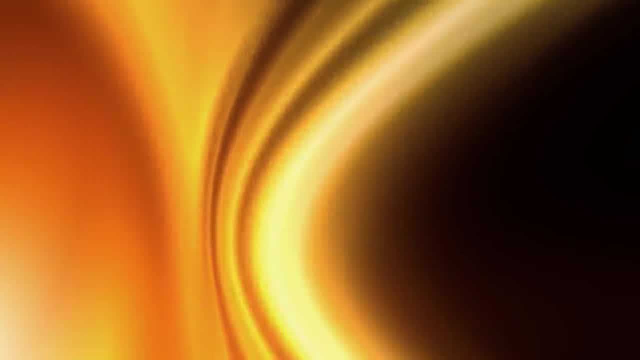 As I was saying at the beginning, it's not possible to state that light is only a particle or a wave. It can be considered as both at the same time. And there's more. This is true, But not only for electromagnetic radiation. 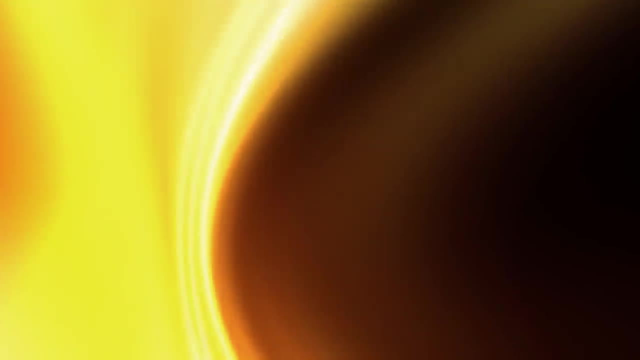 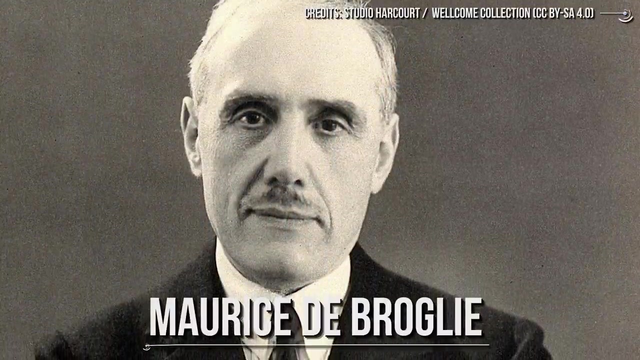 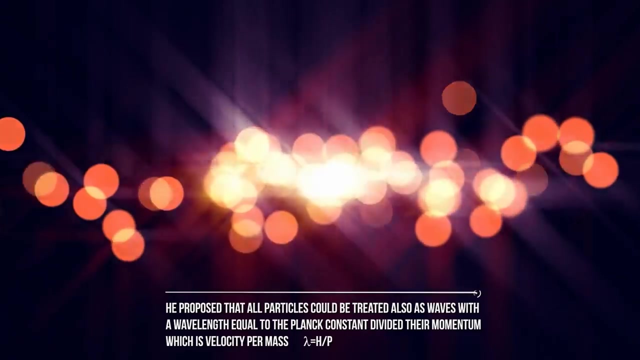 Physicists have discovered that the same behavior of light is proper of all matter: The wave-particle duality of matter. In 1924, the famous physicist de Broglie tried to reverse the relation discovered by Einstein. He proposed that all particles could be treated also as waves with a wavelength equal to the 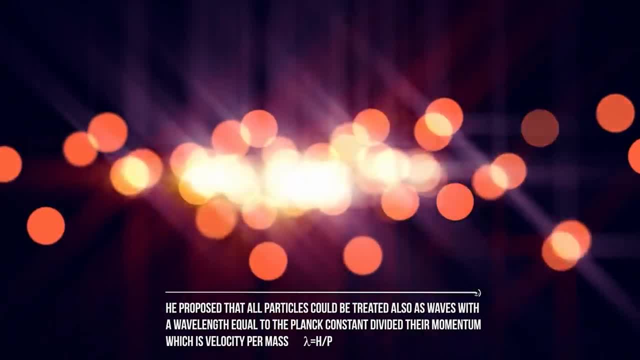 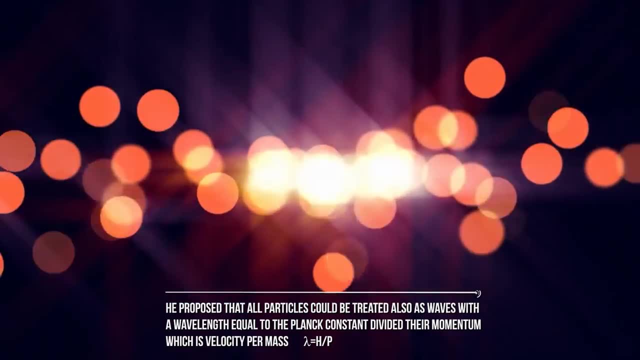 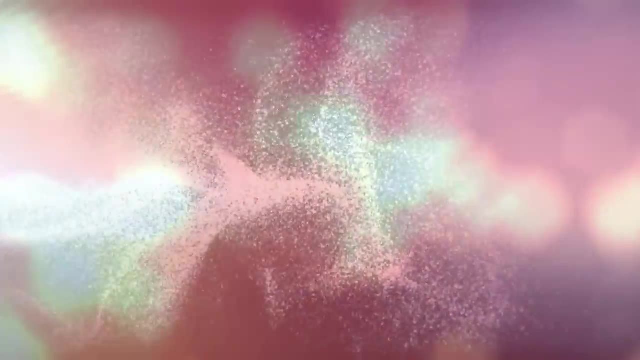 Planck constant divided their momentum, which is velocity per mass Lambda, equals h divided by p, Where h is Planck's constant and p the moment. This hypothesis was then proved by Davison and Germer, who realized a very important experiment. They fired a beam of electrons against a nickel target and they observed that the particles 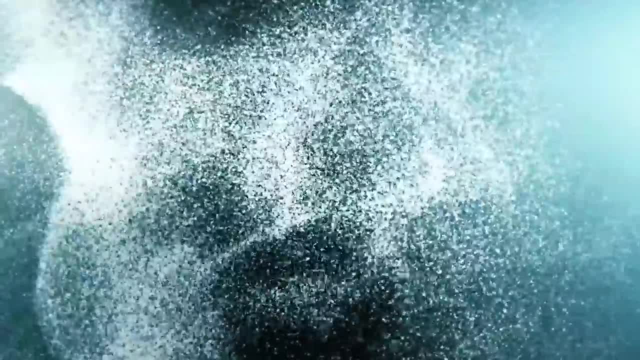 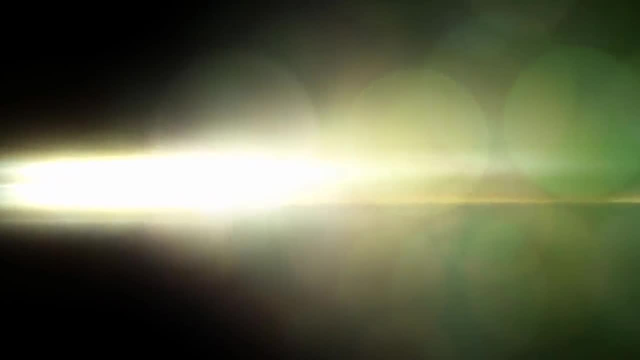 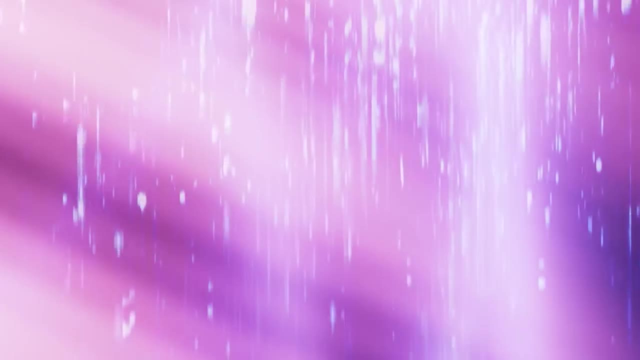 were scattered with the same diffraction pattern of light. Absolutely crazy. But why does nature behave like that? To understand this, we need quantum mechanics. In this extraordinary theory, Each particle is linked to a wave function. The square of this function represents the density of probability of finding the particle. 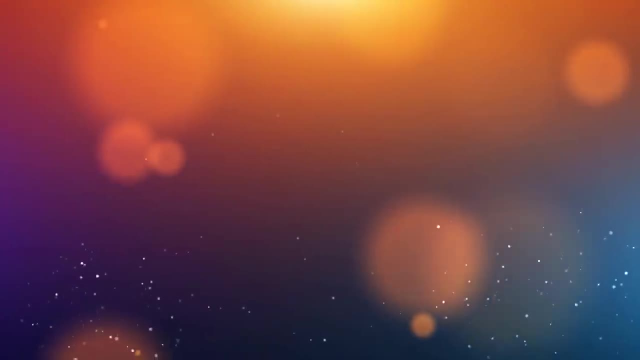 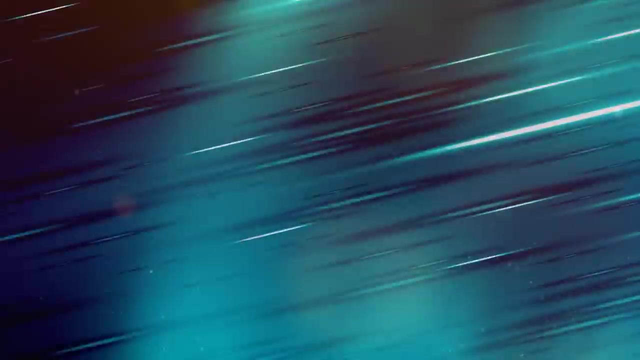 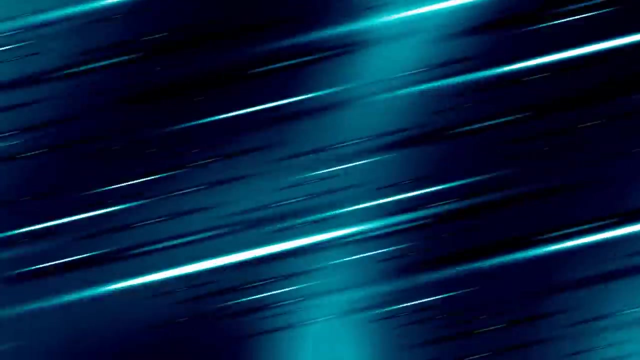 on a particular point. So particles are not waves, but they behave following a wavy function that is linked to the probability of observing them in space. This is also the concept under the uncertainty principle of Heisenberg, that states that the product of uncertainties in the position and the momentum, which is linked to wavelength, 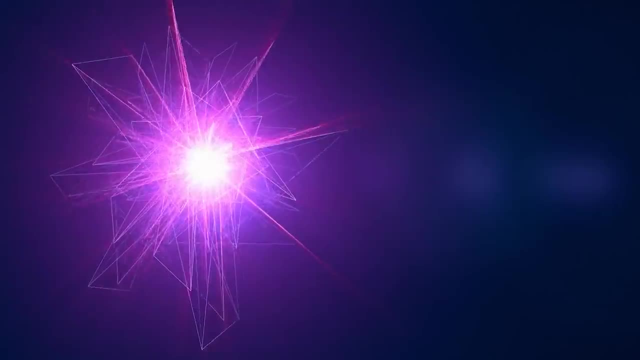 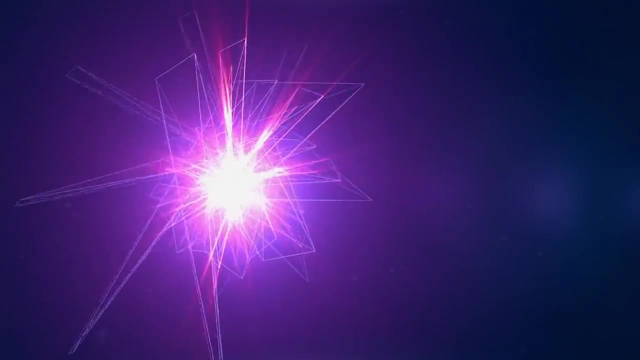 must be higher than a constant value. If one of these quantities is very precise, the other is totally uncertain. And here is the wave-particle duality explained in a few words. When we consider an object as a particle, position is relatively well defined.